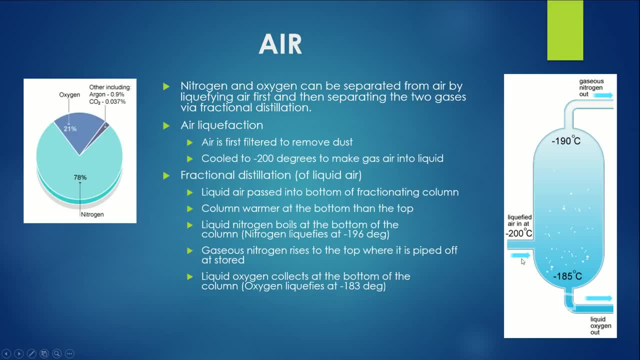 And we can see that because the entering temperature is around 200 degrees negative and you've got negative 185 at the bottom and negative 190 at the top, so the bottom is warmer. So what happens is because nitrogen liquefies at negative 196 degrees. 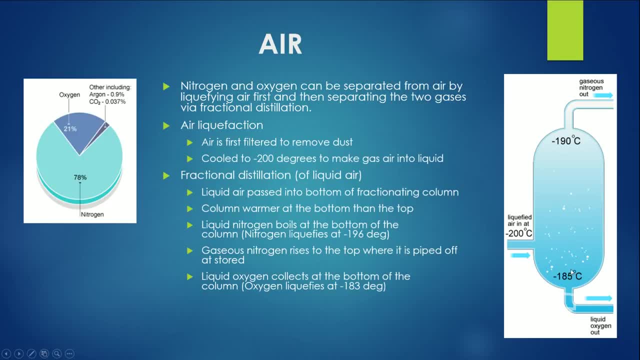 the bottom part here, which is negative 185, is way too too hot. What that means is that the liquid nitrogen that comes in with liquid air will actually boil down at the bottom and it will rise to the top, where gaseous nitrogen is taken out and stored. 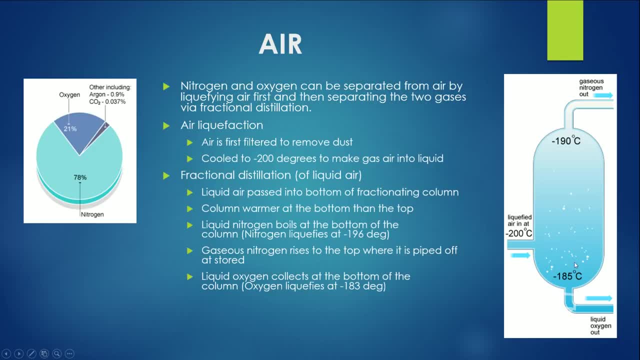 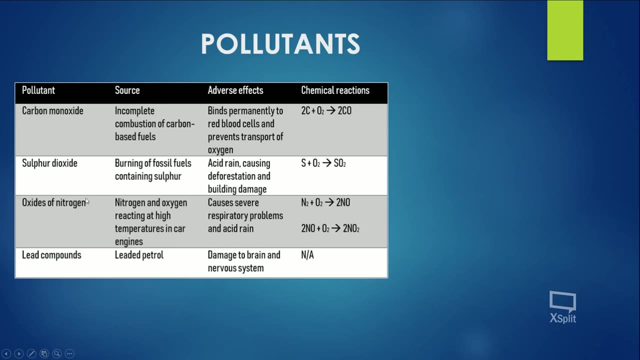 The bottom part, oxygen. the liquid oxygen can be sort of piped out down at the bottom and that's, you know, pretty simple and we can store that. So we've essentially separated nitrogen and oxygen. as simple as that. The pollutants of air mainly are carbon monoxide, sulfur dioxide. 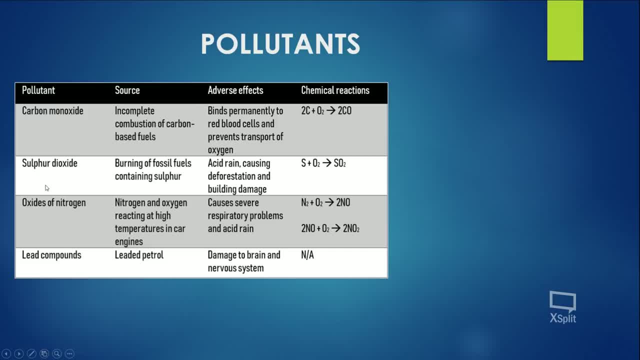 oxides of nitrogen and lead compounds, and you need to know the sources of these pollutants, along with how it can affect our body and the environment. basically So, carbon monoxide is caused or produced from the incomplete combustion of carbon-based fuels. 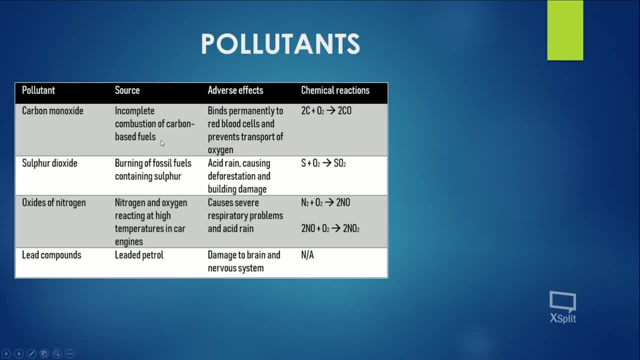 So normally, if you burn carbon and sufficient oxygen, you'll actually form carbon dioxide, And incomplete combustion, for example, when you don't have enough oxygen- you'll actually form carbon dioxide- carbon monoxide instead of carbon dioxide. So carbon monoxide is detrimental to our health. 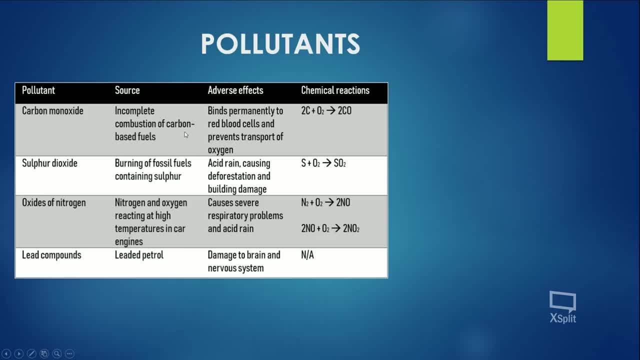 because it binds permanently to red blood cells and the red blood cells normally carry oxygen. so basically, the carbon monoxide prevents the transport of oxygen and that can lead to serious problems. So here is the chemical reaction that is relevant to that. Sulfur dioxide is formed by burning fossil fuels which contain sulfur and the sulfur. 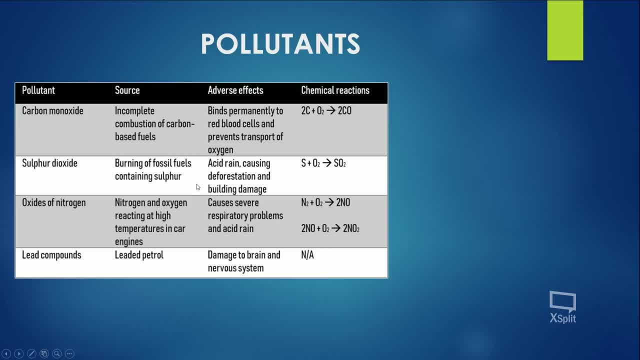 California call acid rain, and that can cause deforestation and building damage and things like that, and so, of course, sulfur added to oxygen will give you sulfur dioxide and this equation- here The oxides of nitrogen- is made when nitrogen and oxygen react at really high temperatures and you find that inside car engines with something called Biting Bear. 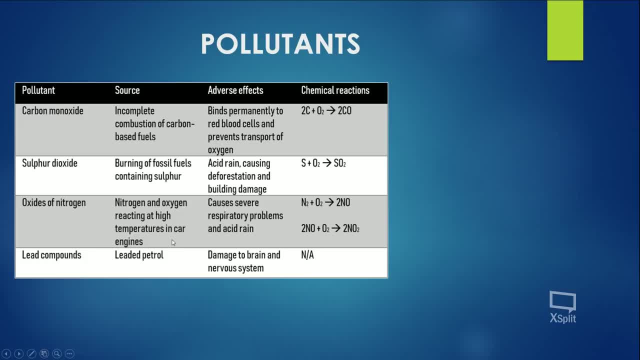 in mind that it's not actually the combustion inside the engine that is causing these pollutants to form. The oxides of nitrogen again is just caused through uncleannesspertty high temperature. This is caused through ar flakesiries due temperatures inside car engines and that causes the nitrogen and the oxygen. 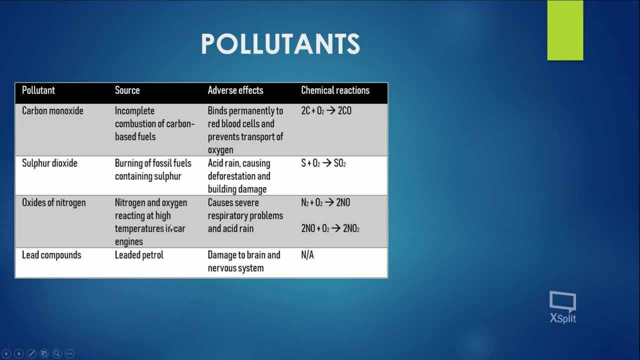 inside the air to to react with each other, and oxides of nitrogen can cause severe respiratory problems, along with the fact that it can also cause acid rain as well. so here are two equations that you should know, for that lead compounds are present in lead petrol, and so ingestion of these things can. 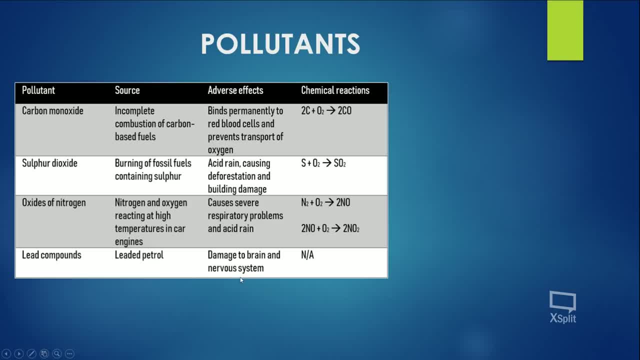 actually damage the brain and have pretty you know bad consequences in terms of what it does to our nervous system in general. so one way to counteract the production of nice Victer catalytic converter. so this is a pretty smart way of sort of neutralizing these pollutants. so basically what it does is that catalyze. 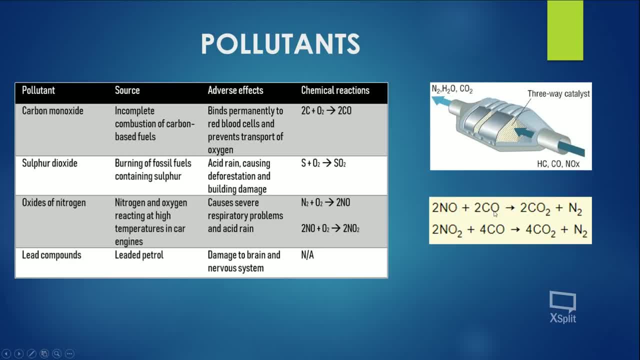 is the reaction between nitrogen oxide and carbon monoxide, producing carbon dioxide and nitrogen, and, as you know, carbon dioxide isn't that bad. it can also cause respiratory diseases. catalyze the reaction between nitrogen dioxide along with carbon monoxide and it forms again carbon dioxide and nitrogen. and this is really smart because it removes two pollutants which 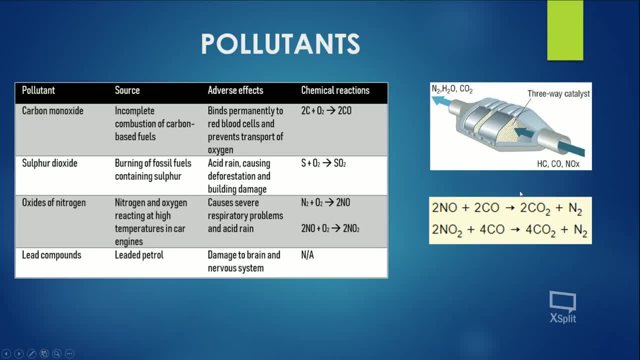 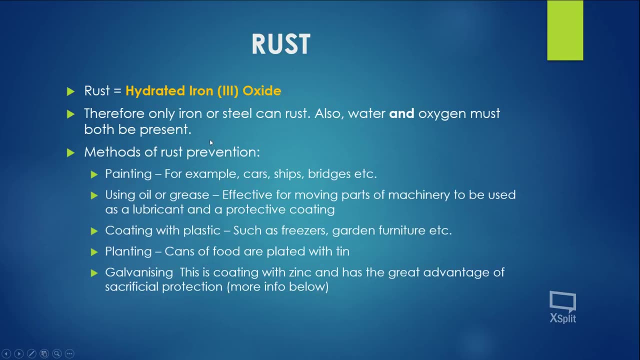 is nitrogen oxide and carbon monoxide at the same time to produce two uh fairly non-harmful elements, or sorry, not elements, just um products. so let's talk about rust, right? so rust is Hijraded iron oxide, its all. that it is so hydrated means there's water and iron oxide. 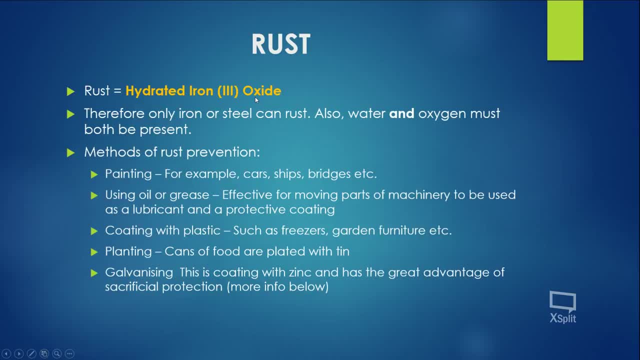 is just simply the product of, or the ionic product of, iron combining with oxygen. so therefore rusting can only happen in iron or steel, because steel contains iron and um, and therefore only iron or steel can be termed rusting. Everything else is technically corroding, right? so not only do you need iron or steel for 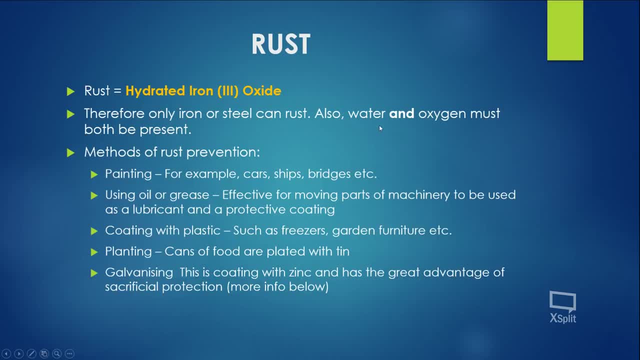 rusting to happen you need water and oxygen, because obviously it's the reaction between iron and oxygen and inclusive of water. so all three things have to be present. so a couple of methods of rust prevention would mainly be to sort of offer some sort of physical boundary so that the iron 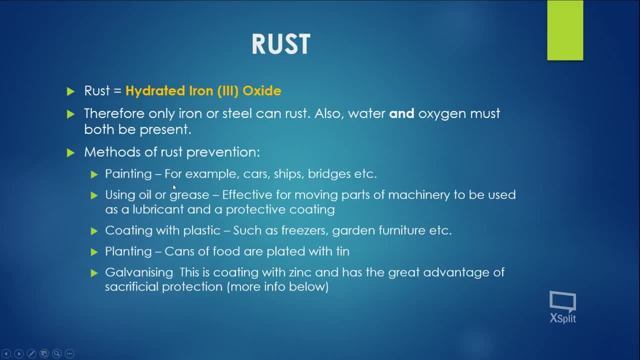 doesn't react with oxygen. so it can be, for example, painting using oil or grease which acts as a coating but also effective as a lubricant. and moving parts of machinery and things like that, perhaps coating with plastic, you know, planting and galvanizing. so galvanizing is important because it offers sort of 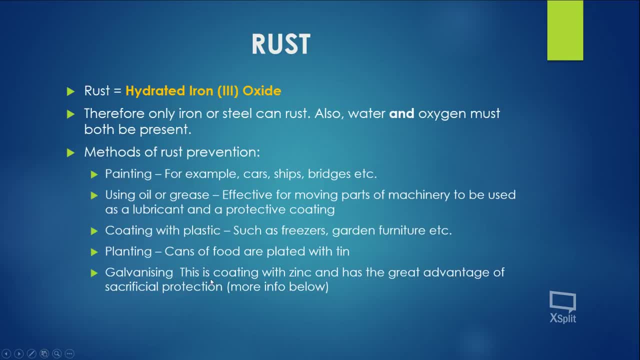 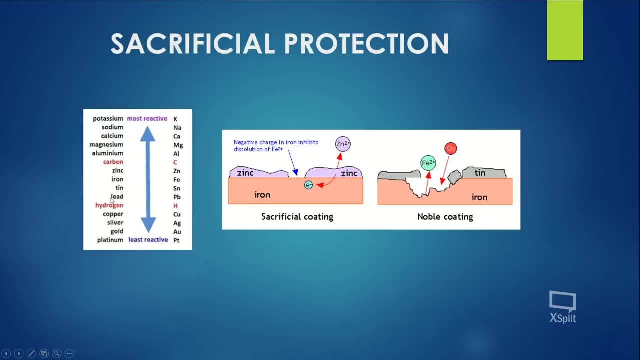 something called sacrificial protection, and we'll look at that in a bit more detail. yeah, so the first thing about sacrificial protection is the idea that there's a difference in reactivity between zinc and iron. well, the first thing about sacrificial protection is the idea that there's a difference in reactivity between zinc and iron. 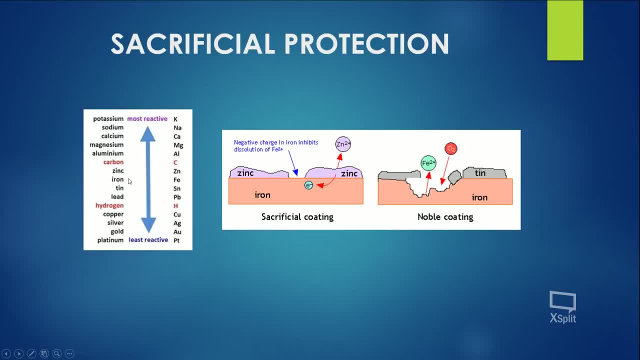 remember, in this reactivity series, zinc is higher up than iron, suggesting that zinc is more reactive, which means that zinc would much prefer to be in its ionic form rather than iron. so that is, higher tendency of zinc to go into its ionic form rather than iron. so what happens is that here, this is the 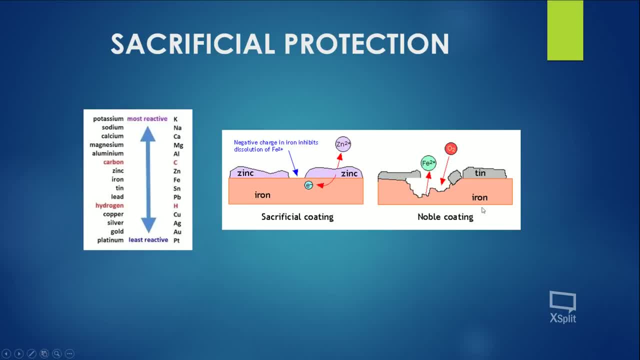 standard coating to the right right. so this is not sacrificial protection and this is just the standard idea that you can coat the iron with tin. but the problem is, when the tin wears off and there's exposure of the iron, the oxygen can easily come and oxidize the iron and so the iron goes from iron element into 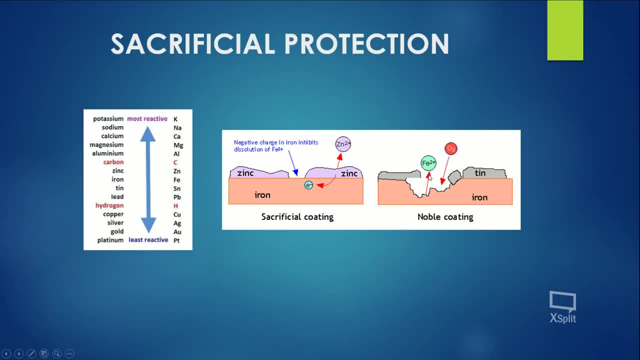 the ionic form, which is iron cations, basically Fe2 plus, and as that happens you start to lose the iron and basically cause rust. now in sacrificial coating, you coat it with zinc rather than tin and of course the zinc is more reactive than iron. so even if you do get a little bit of hole forming and the 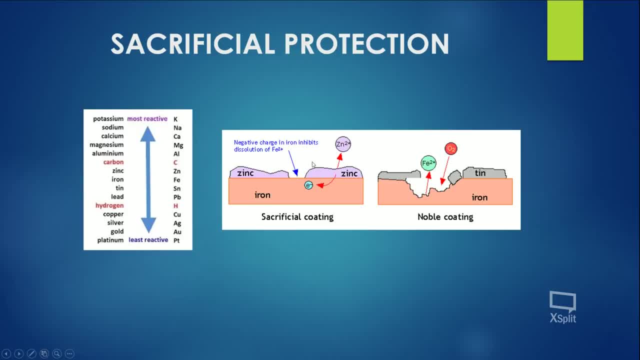 breakdown of the zinc coating, what will happen is that the oxygen doesn't oxidize the iron, but it actually reacts with the zinc instead, remember, because the zinc is more reactive than iron. so, rather than the iron corroding or rusting, the zinc will take its place. therefore, it sort of sacrifices itself for the iron. 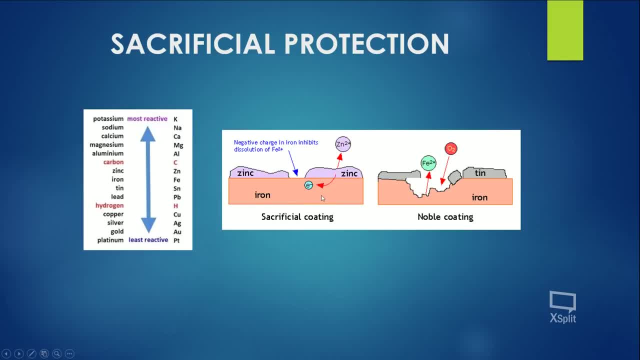 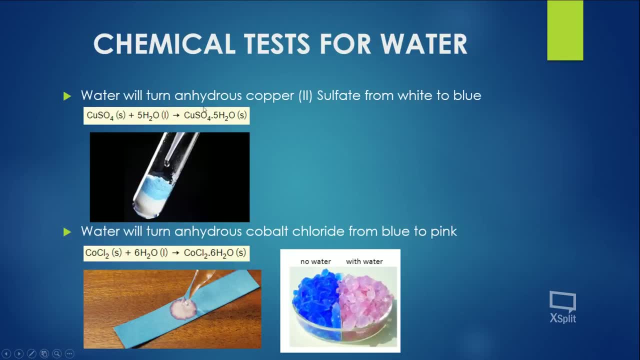 and therefore you don't get as much rusting going on. so here are some chemical tests for water, right? so water will basically turn anhydrous copper sulfate from white to blue. so here is the reaction: you got copper sulfate, which obviously does not contain any water, which is the anhydrous form. you add that